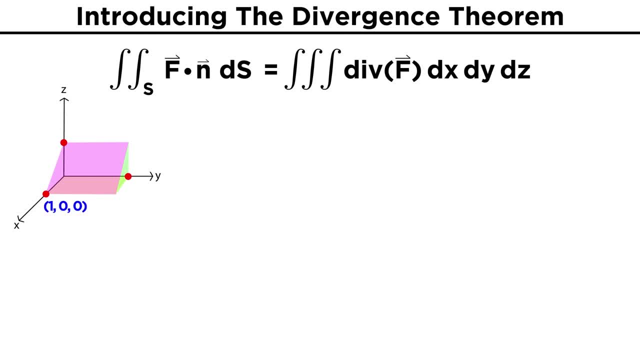 Consider the surface of this triangular prism, which occupies x from zero to one and y from zero to two. It has a flat base in the xy plane and the top surface is given by the plane. z equals one minus x. Now let's say there's a vector field in this space which is given by F equals. 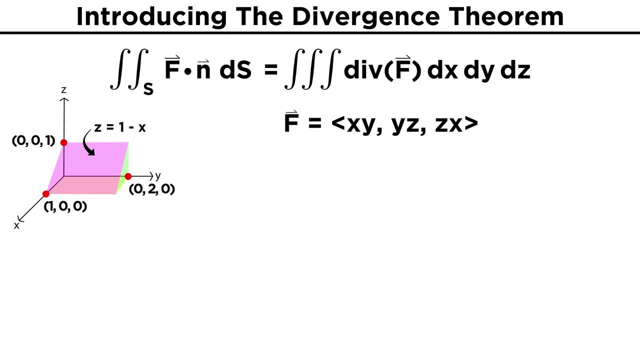 xy, yz, zx. If we wanted to calculate the surface integral of this field over the surface S without using the theorem, we would have to split each of the five flat surfaces of the prism into their own surface integrals and calculate each individually. 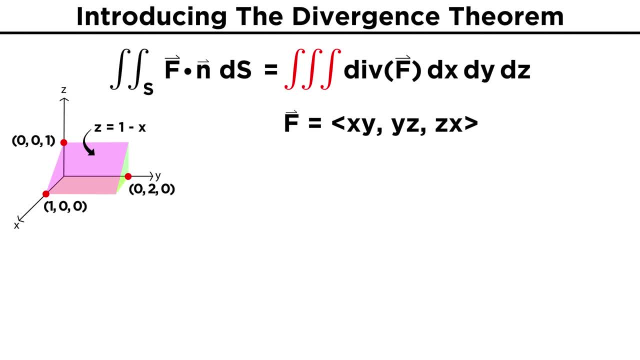 Luckily the Divergence Theorem reduces our problem. It reduces our work to one triple integral over the region of the prism. The Divergence Theorem states that the surface integral will be equal to the triple integral of the divergence of F over the region. so first let's find the divergence of F. 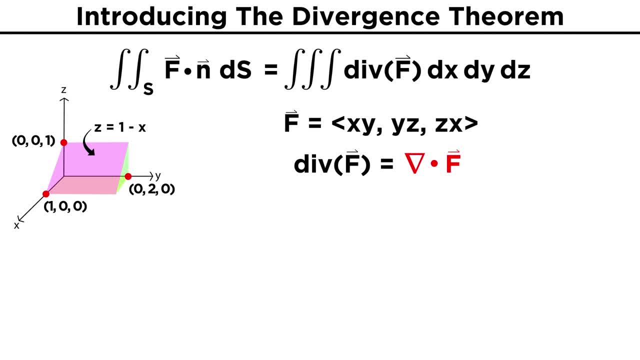 Recall that the divergence of a vector field is delta dot F. where delta equals ddx ddy �ツ. K case, the divergence will be: del dot F equals Y plus Z plus X. Now we have the divergence, but before integration we must get our bounds sorted out. 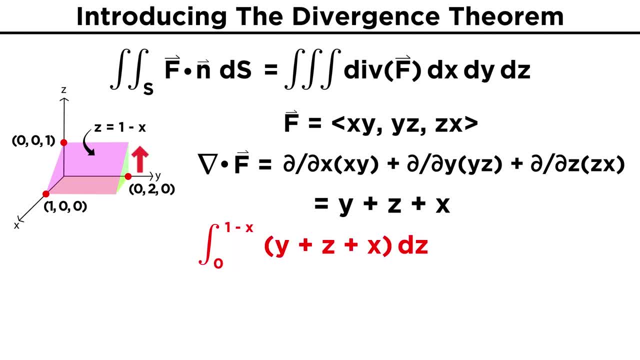 We get these from the region of our prism. One simple way to express these bounds is integrating Z first, letting it run from zero to one minus X. Now we don't have any more complicated bounds, so we can integrate Y from zero to two, and 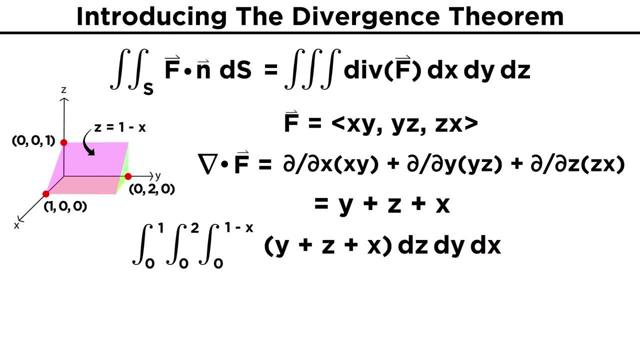 X from zero to one. So our integral ends up being the integral from zero to one, the integral from zero to two, the integral from zero to one minus X, of Y plus Z plus X, DZ, DY, DX. Integrating Z first, we get YZ plus Z squared over two plus XZ. 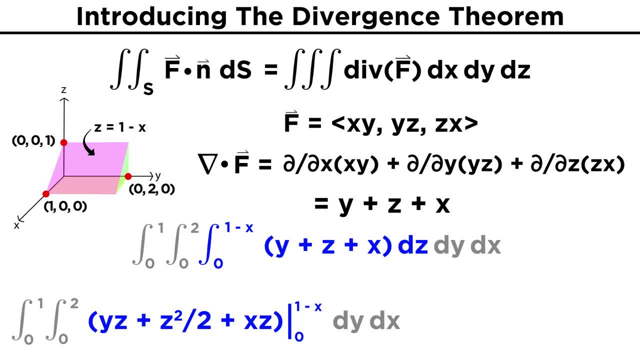 Where Z equals Y plus Z squared over two. we get YZ plus Z squared over two plus XZ. Where Z is evaluated from zero to one minus X, Factoring out a Z and evaluating, we get one minus X, Y plus one minus X over two plus. 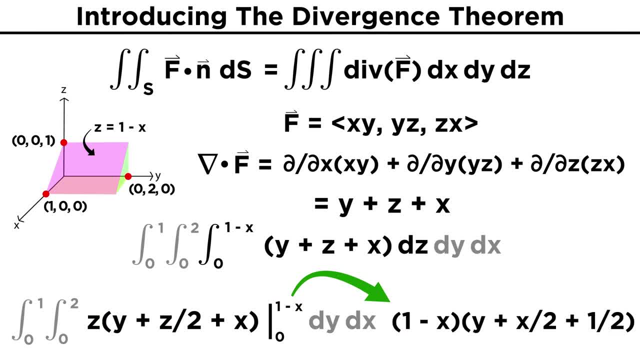 X, or simplifying the X terms: one minus X, Y plus X over two plus one half. Next, we must integrate with respect to Y, which gives us one minus X, Y squared over two, plus XY over two, plus Y over two, where Y is evaluated from zero to two. 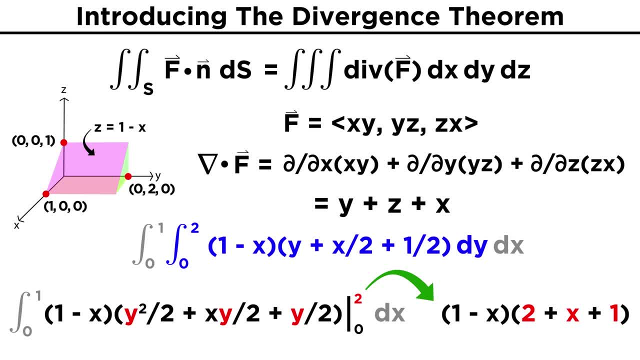 Evaluating this, we get one minus X times two plus X plus one, or just one minus X times X plus three. Now if we multiply this out, we get the integral of X plus three minus X squared minus three X DX. Simplifying gives us three minus two X minus X squared. 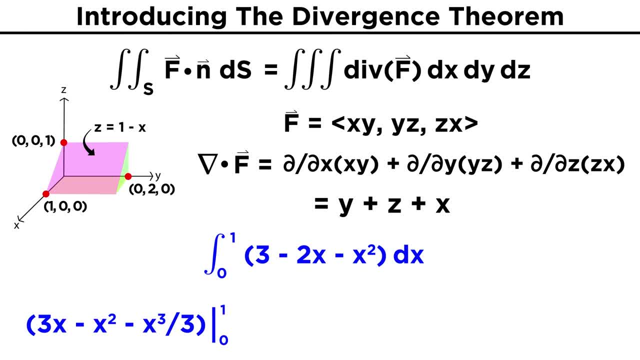 Integrating we get three X minus X, squared minus X, cubed over three, where X runs from zero to one. And finally, evaluating gives us three minus one minus one third, simplifying to five thirds: This is the value of our surface integral, which we used the divergence theorem to calculate. 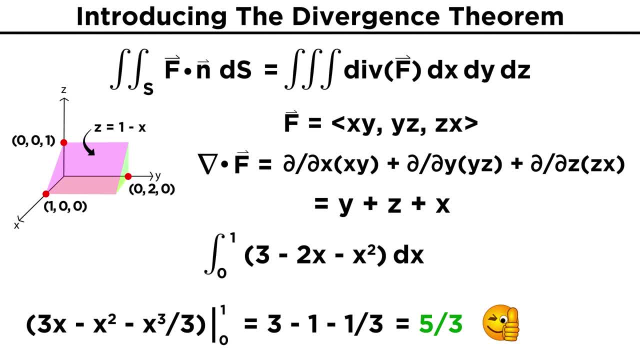 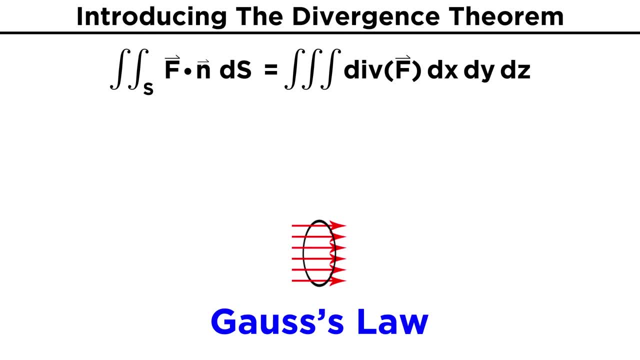 The divergence theorem is another useful tool for calculations and it has a variety of applications. In fact, the theorem is used in Gauss's law to relate the flux of an electric field, which would be the surface integral part of the theorem, to the amount of charge contained. 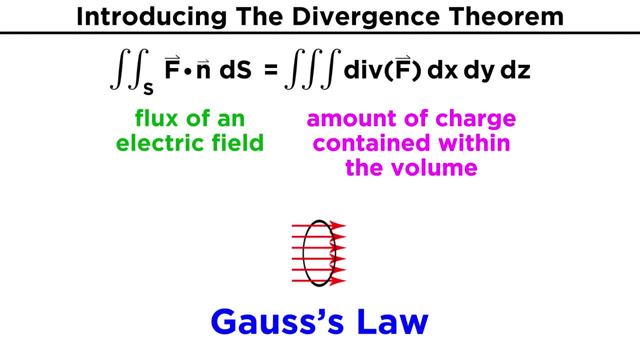 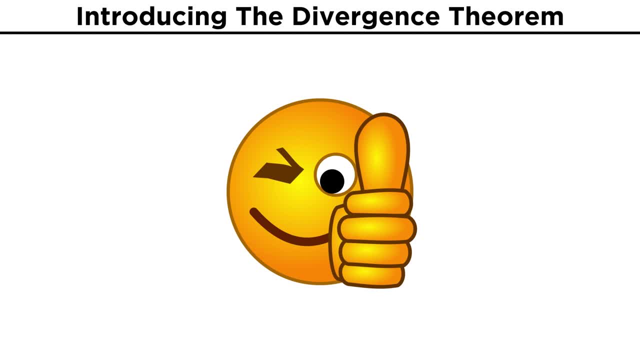 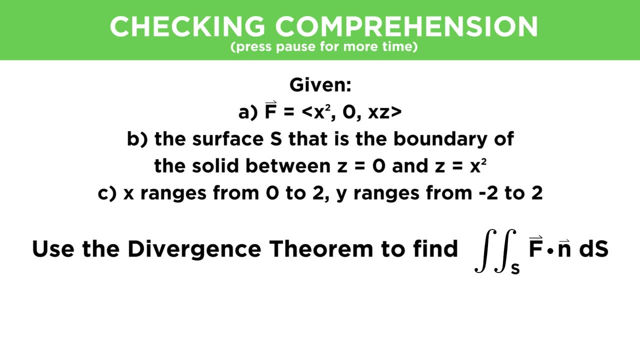 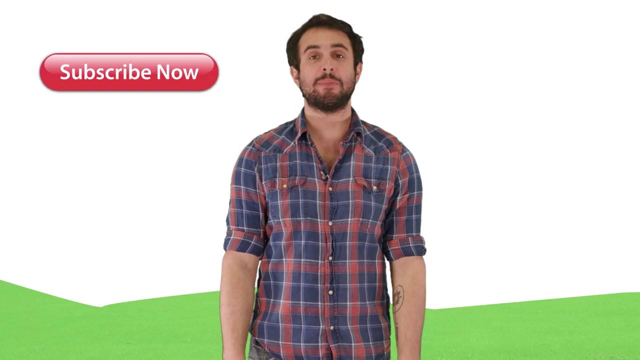 within the volume, which would be the triple integral part of the theorem. And with this we've wrapped up another series of experiments. But before we go on to more advanced topics, let's check comprehension. Thanks for watching, guys. Subscribe to my channel for more tutorials. 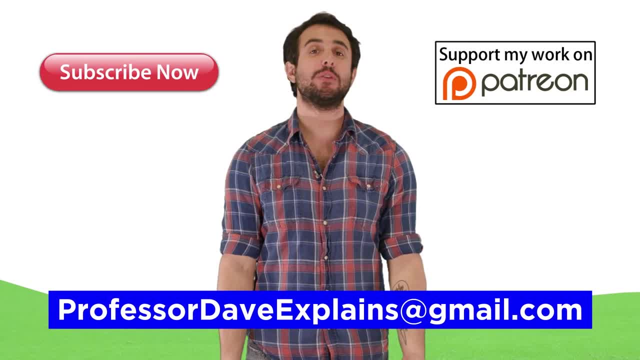 Support me on Patreon, Twitter and Instagram. I'll see you next time. Thanks for watching and, as always, feel free to email me professordaveexplains at gmailcom.